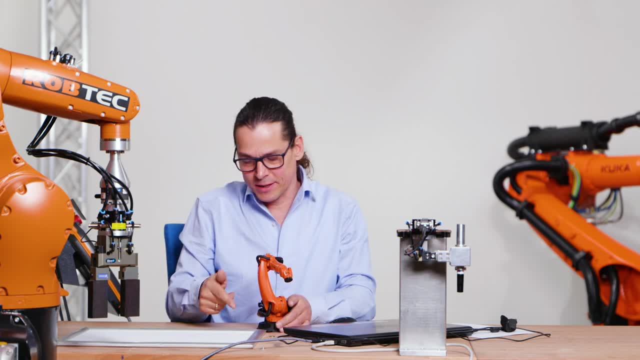 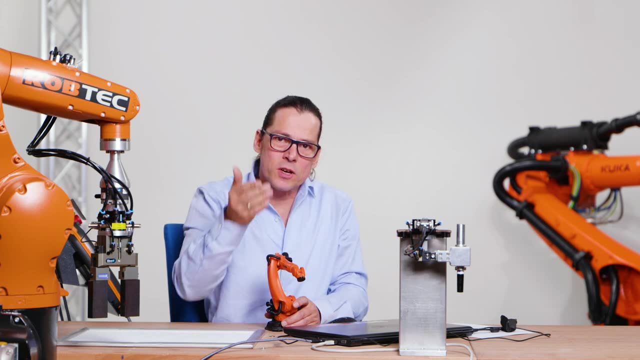 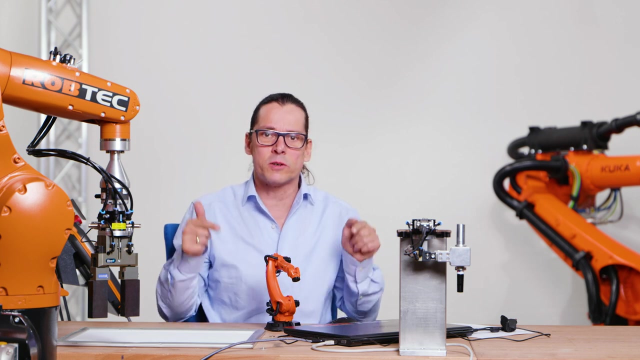 video and the world coordinate system, and this is here located. if you move, set plus, the robot always moves to the top. this is very, very, very important. for example, you have on crash and you don't know where the coordinate systems of this robot are defined. here you use that coordinate system because on every robot 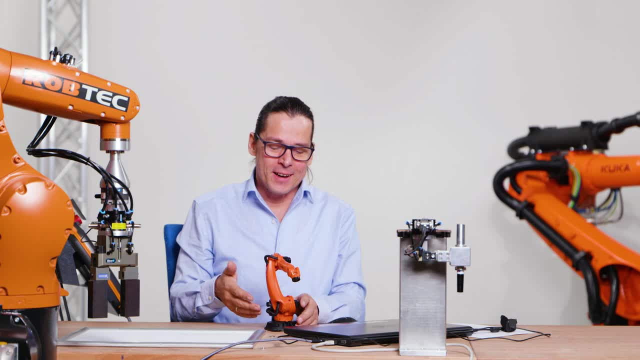 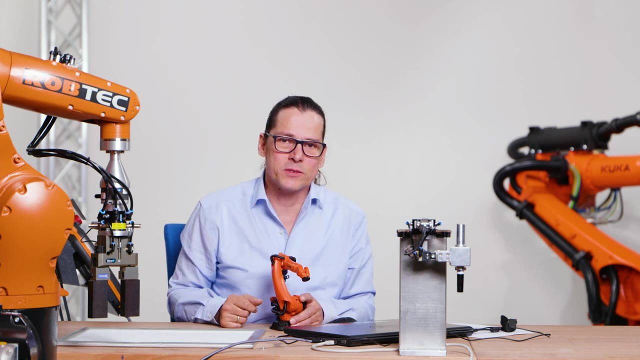 it's the same. you know you cannot change the world. yeah, the world coordinate system means here's the origin, X plus is here, Y plus Z plus. so if you have a problem with your robot and don't know how to move the robot, remember the world coordinate system. 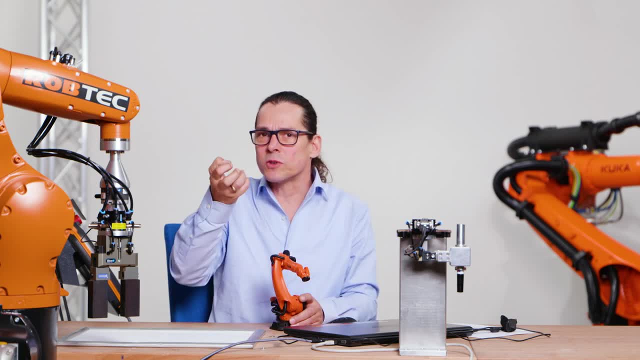 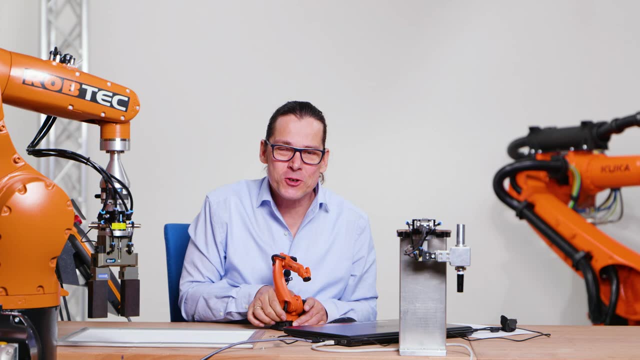 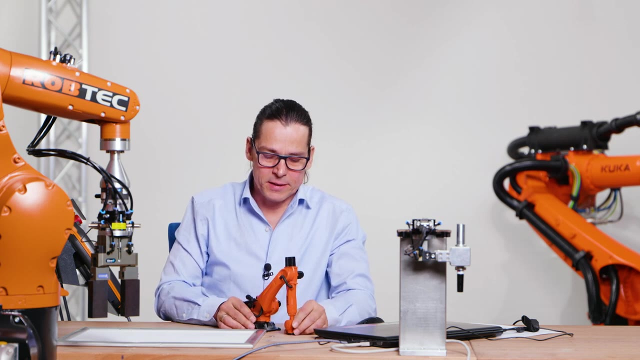 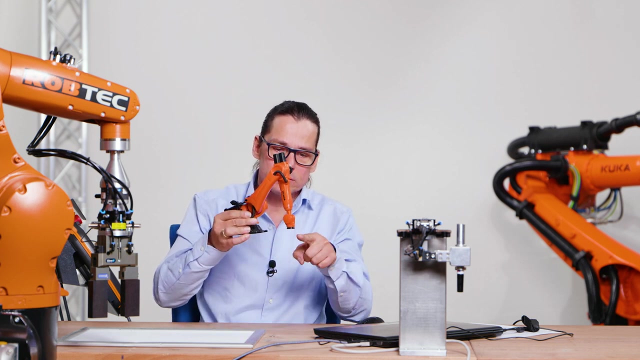 system and move the robot into the right direction, to move the robot away from, example, from a crash. okay, so let's show this on the real robot how this works. for example, the set. i always explain it here. if i down here below, with axis set and the same level like axis one, 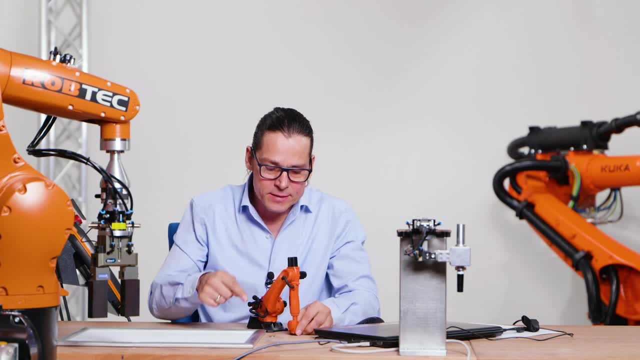 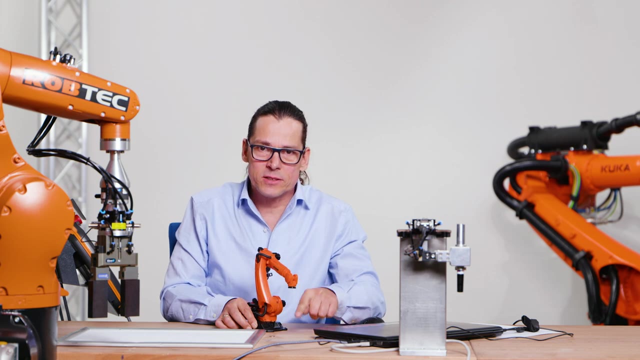 okay, and then the set coordinate here is zero. yeah, it's the same level, uh, like here and when i move now set plus, for example, one meter, then in the set axis is 1000 millimeters. yeah, and the robot counts: here are i am in set 1000 millimeters in this case. uh, it's also in. 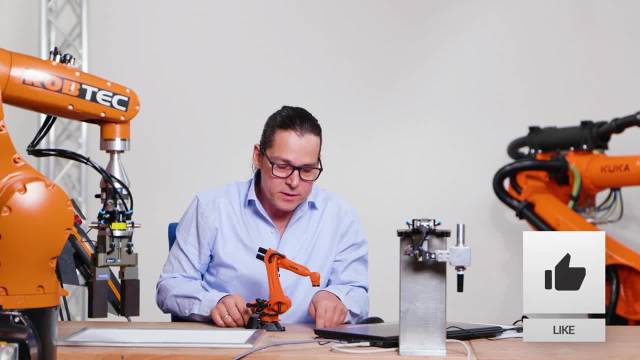 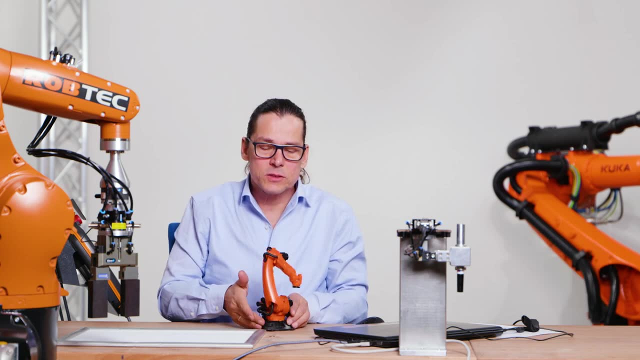 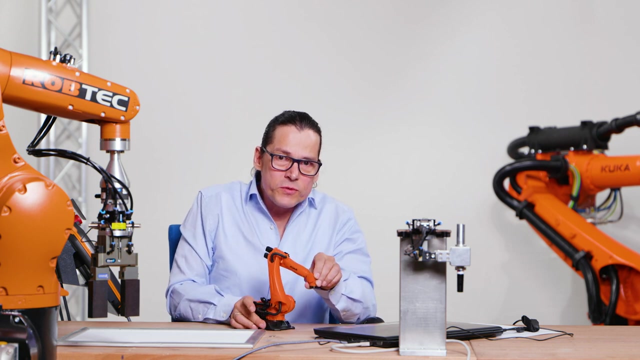 x, for example. or this would be one meter in x, one meter in z and x is y is in the middle. so the coordinates, uh, the robot shows where his x is six here is is in x, 1000. it's that 1000 when i move? 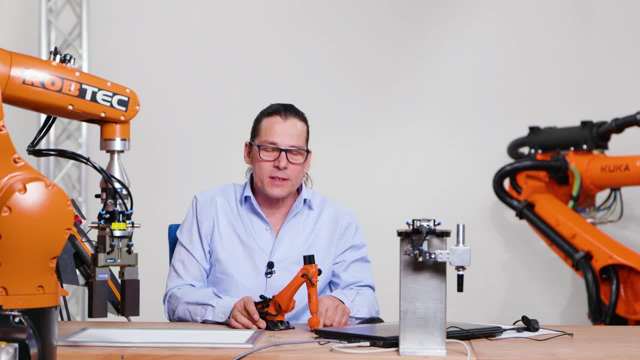 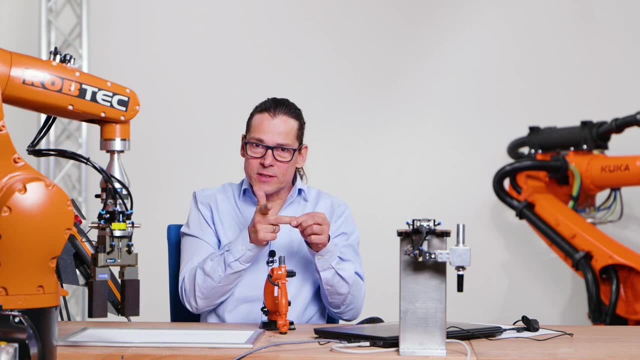 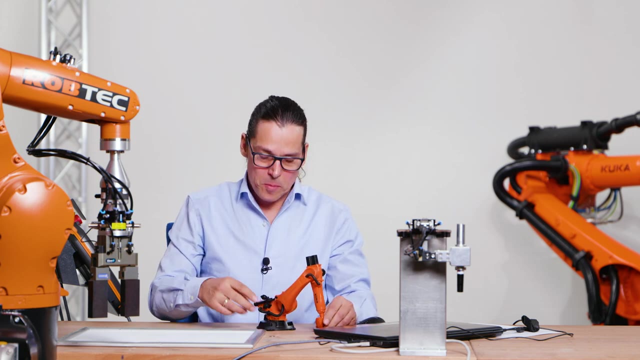 down it's x, 1000 and set zero. when i want to say the robot move to the left. left is that direction. this means y. if i go there now, the coordinates are set zero, y is one thousand and x is one thousand. okay, i hope you understand this. i show this: uh, on the robot again. um, if it's not completely clear, so here: 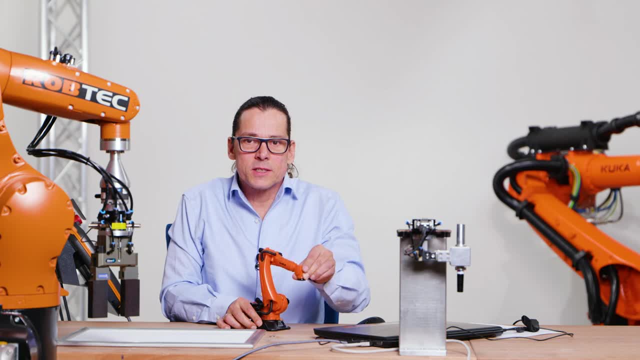 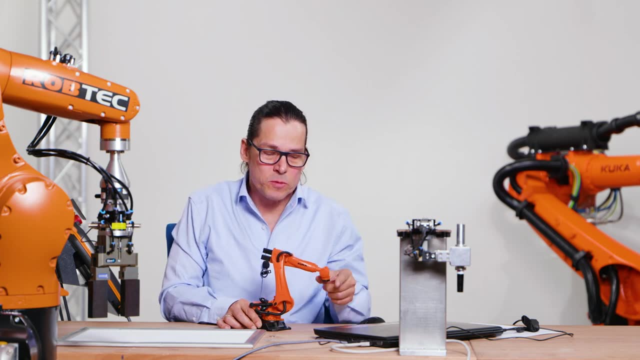 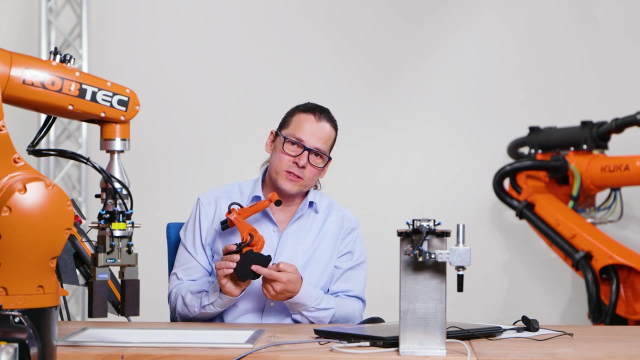 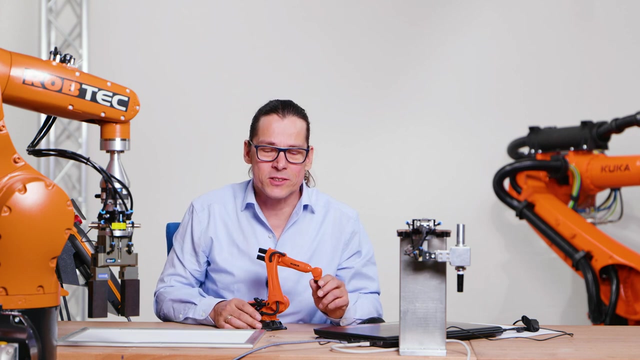 is set zero, set one thousand, y zero, y, 1000, okay, and the robot always counts the difference between x is six now- and the world coordinate system, which is located here, and that's how the robot counts and knows where he is. simple, isn't it? yeah, okay. 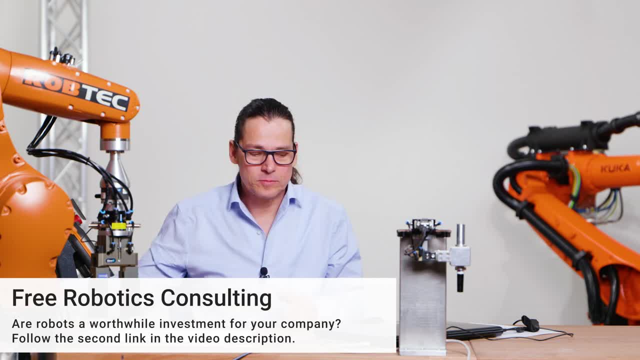 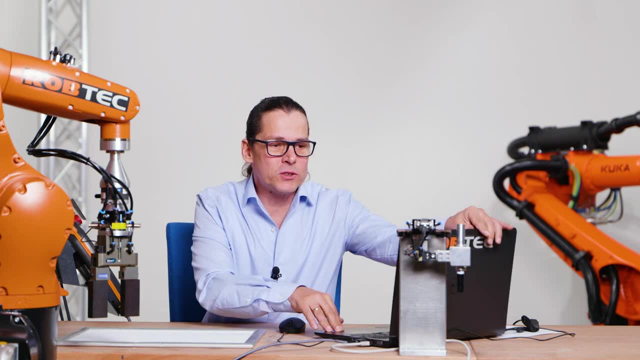 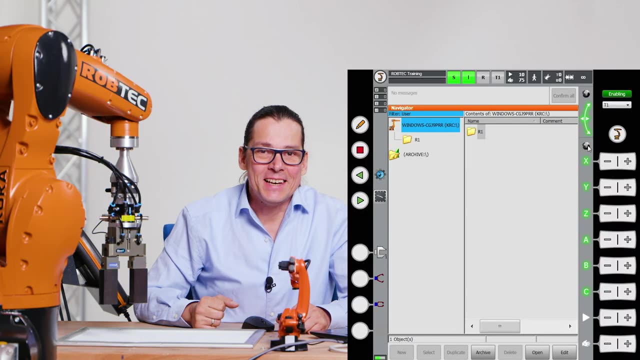 this on the real robot. To show you what button I push, I use my virtual teach panel where I can control this robot. Okay, let's have a look how the robot shows his own coordinates in his teach panel. So for that I go in KUKA on the. 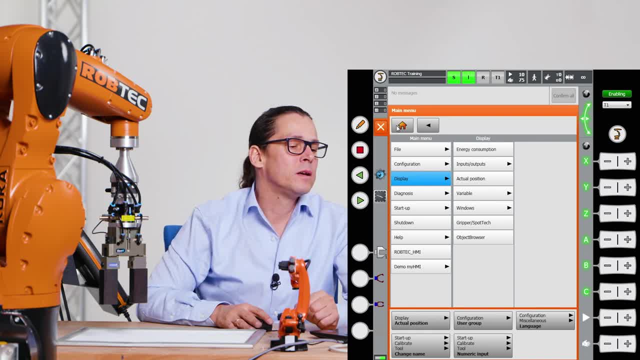 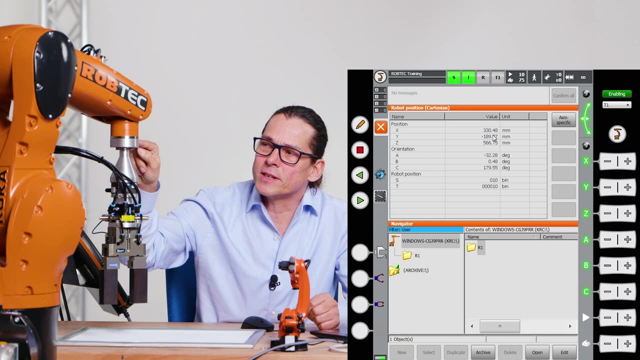 KUKA sign, which means it opens a main menu. I go in the house- This is the first level of the main menu. I go to display and actual position and now, when I selected here the world coordinates, I see the difference between here, axis 6: 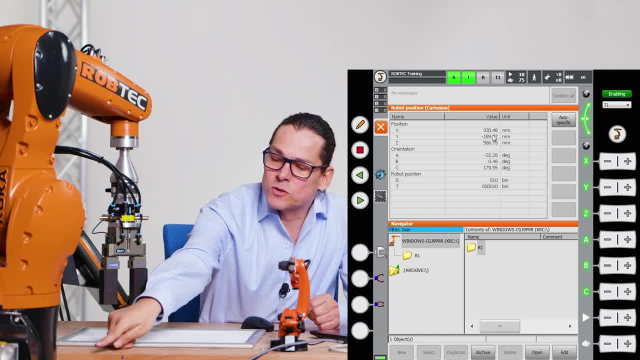 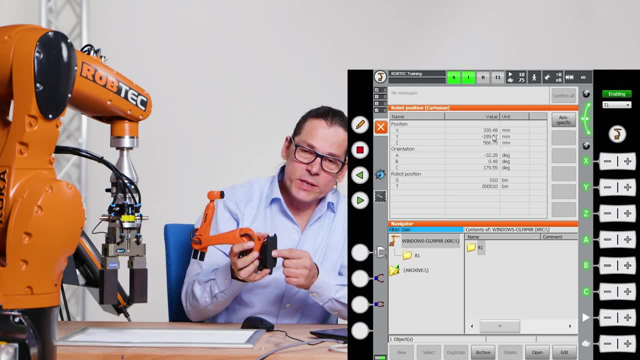 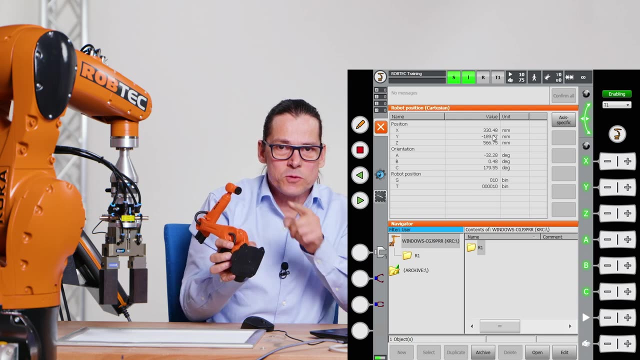 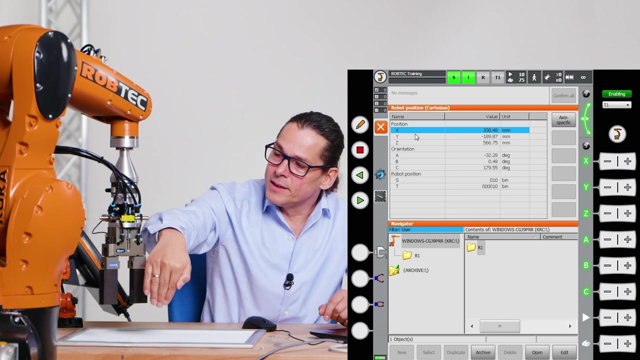 0 in the middle of axis 6 and the world coordinate system. here. I'll explain here The tool is the world coordinate system, here The difference between here 0 0, 0, the world coordinate system and here, axis 6.. This is what it shows us now here as a coordinate in X. this robot is from here. 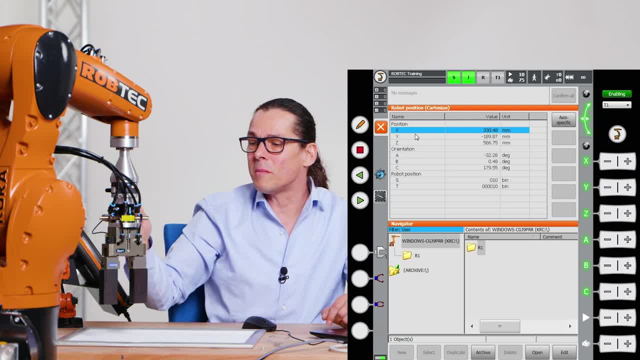 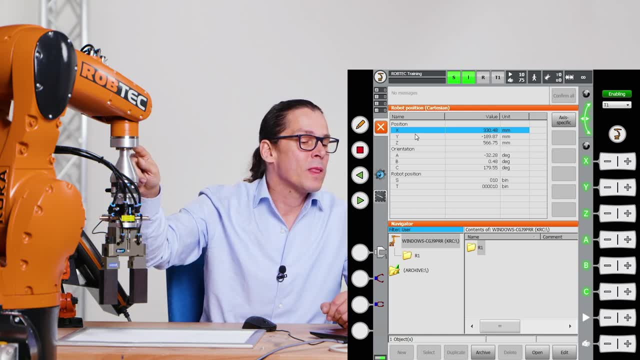 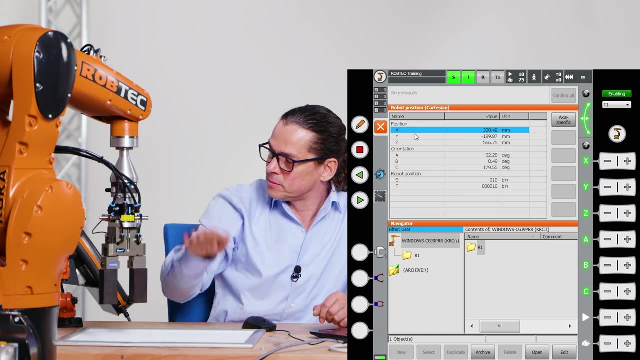 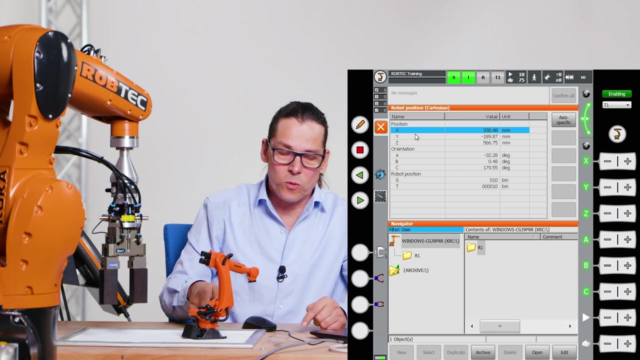 to here, 330 in Y minus. you remember: Y plus is in that direction, Y minus is that direction is 189 and in Z is that 500.. Six, Six Mm Millimeters away from here, down here below 500 here. 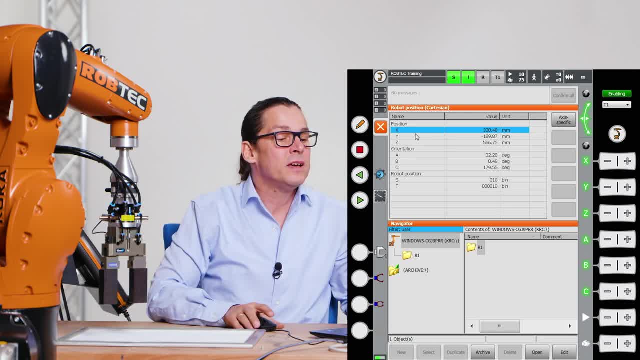 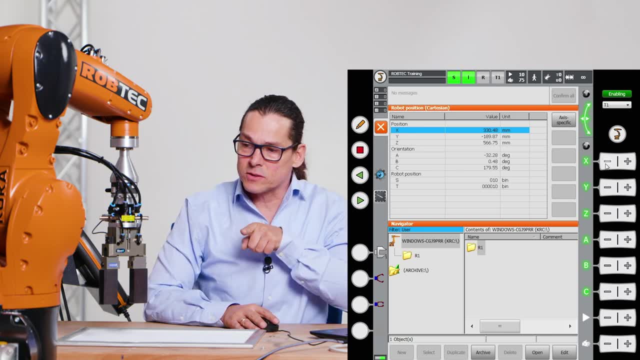 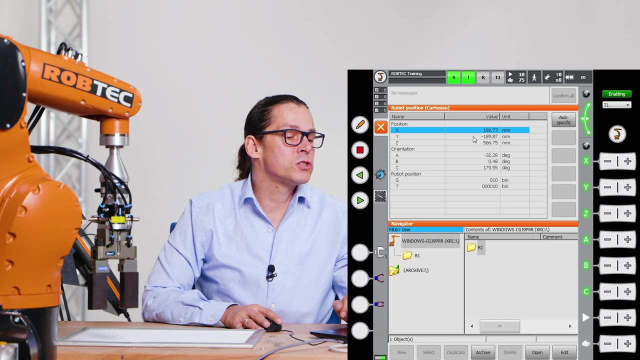 X 330 here and y minus 189.. Let's give it a try. When I, when it moves the robot, So I move the robot in X minus, That means the robot moves in that direction. and have a look What happens here. 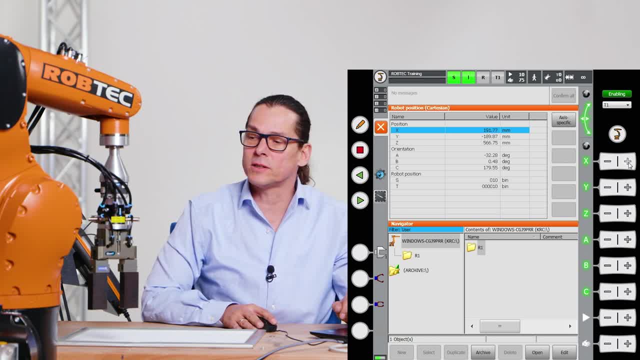 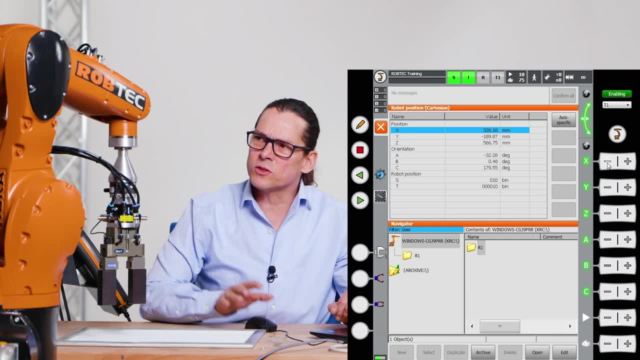 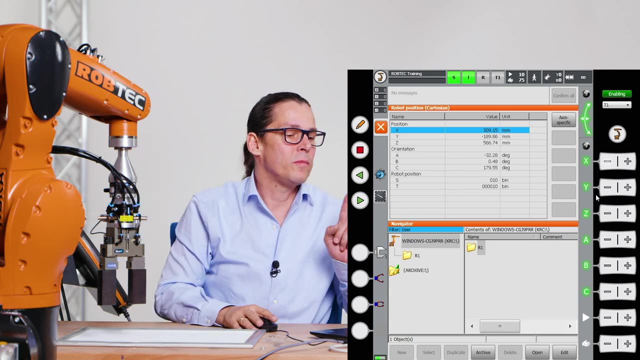 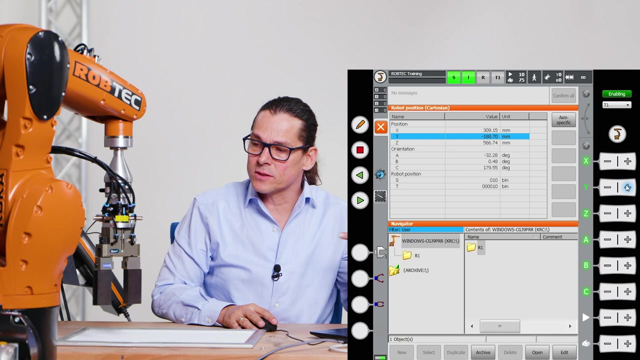 the coordinate Y is now. Now we have 191.. I move to plus and Robert moves here to 385 and he always shows the actual coordinates from axis 6, the middle, This direction. Now I move coordinate system in Y, Y plus goes in that direction and I 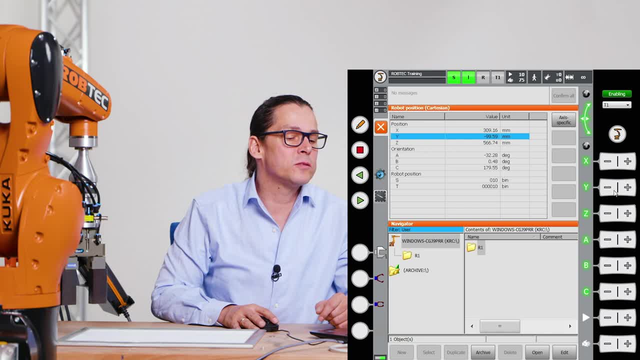 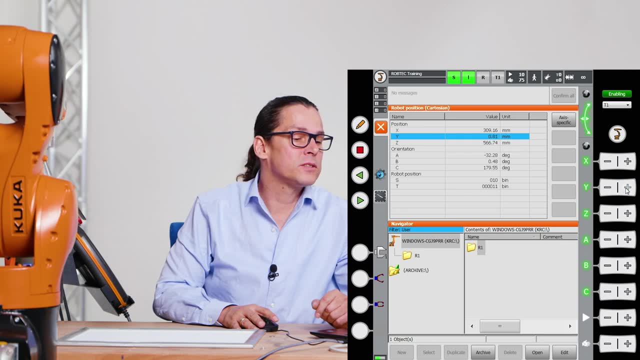 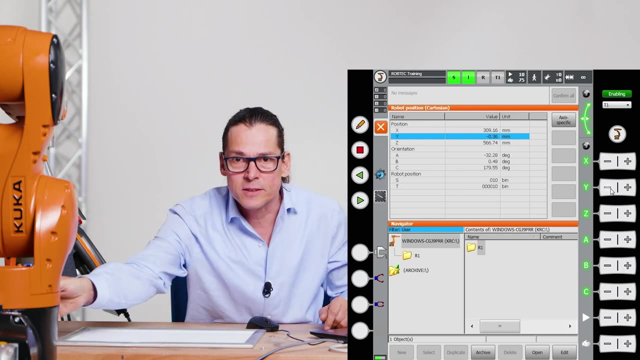 see now the values changing to there. When I'm exactly in the middle, it should be 0.. You see, now I'm exactly in the middle because the coordinate system's origin is exactly here, in the middle of axis 1.. Y is here. I cannot move down here. 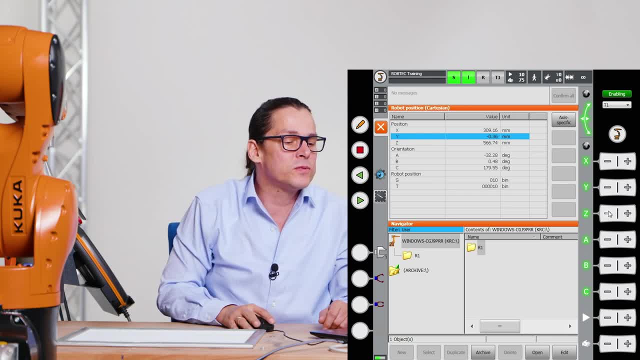 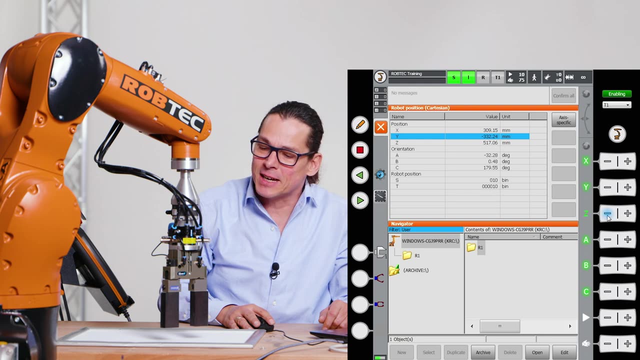 below to 0 in set. but I move as much as I can to 0 in set. but I move as much as I can to 0 in set. but I move as much as I can here. oh, we show you 0 here Now I move down. You see, it changes the set. 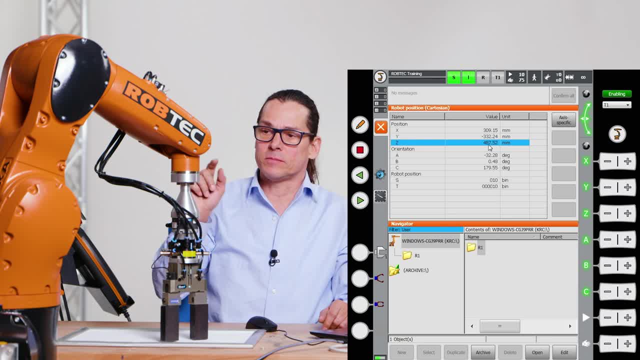 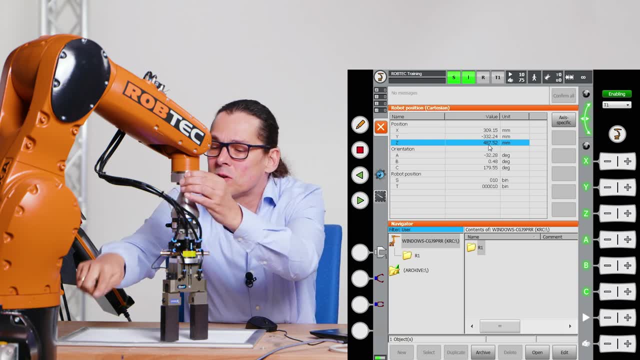 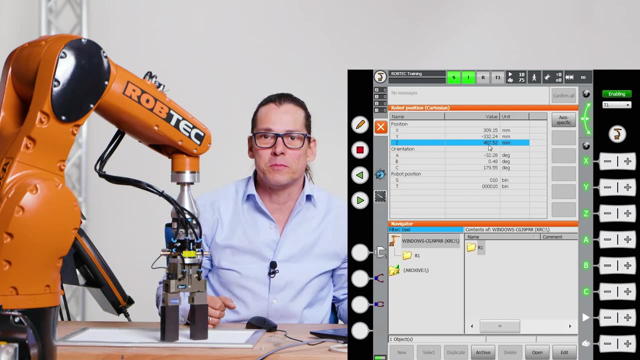 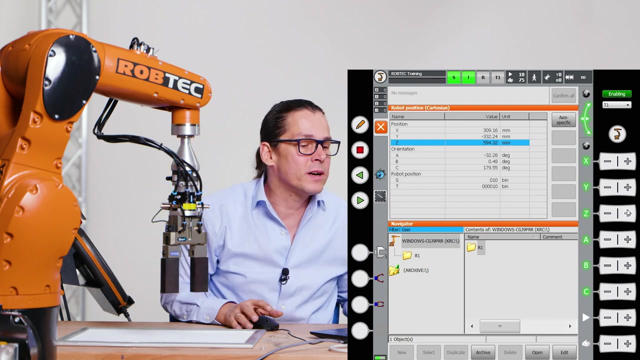 axis, Now it shows 487.. And what does that mean? It does mean here, X axis 6 is 0, up, to X is 1 is 0.. zero is 487 millimeters. that's how the robot counts if i go set to plus, for example, 100 millimeters. 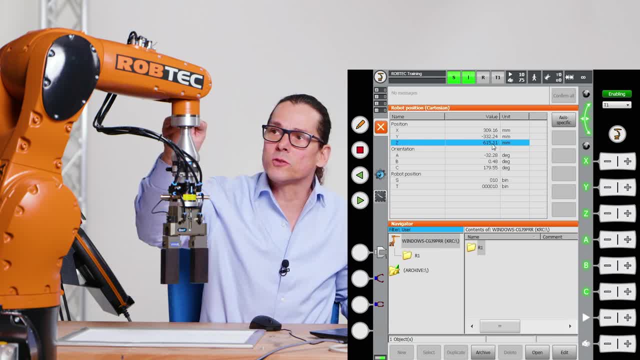 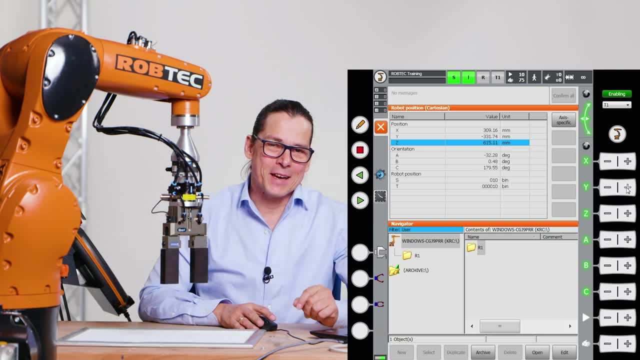 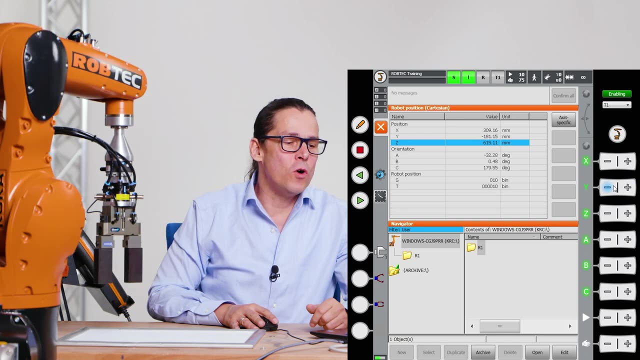 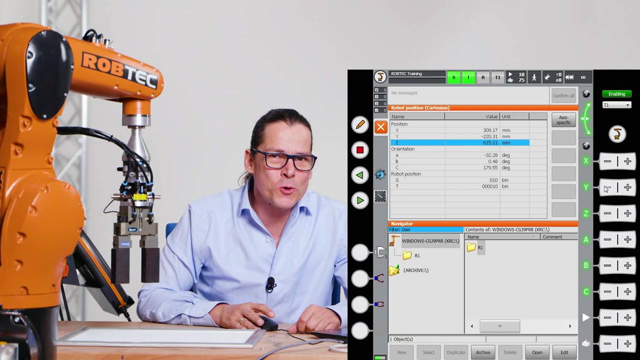 it counts here always the actual position to that. okay, do you understand that? it's very important? okay, i hope you understand now how this world coordinate system, um, works. yeah, if yes, please give us some up, and if you don't understand, write down a comment below i will answer it. 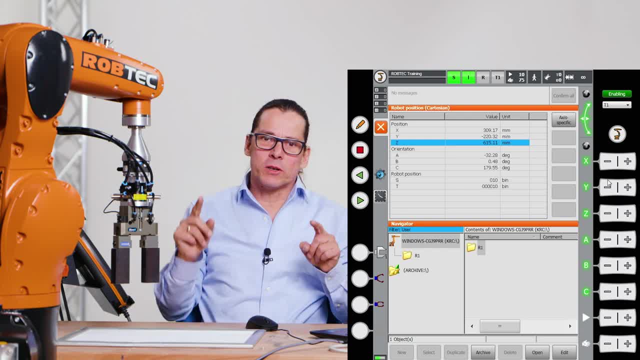 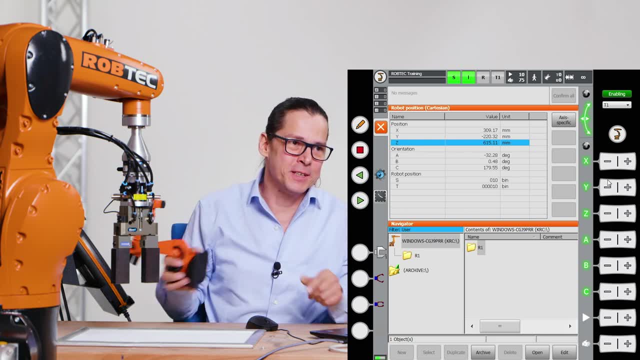 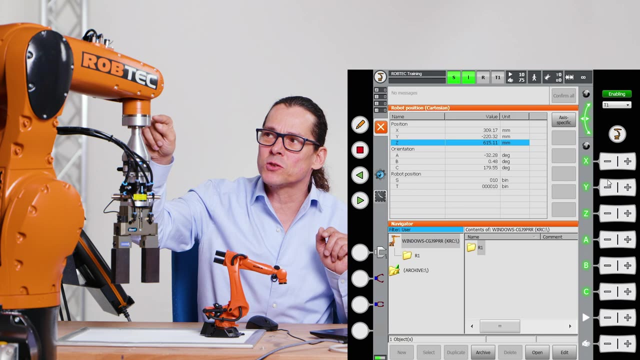 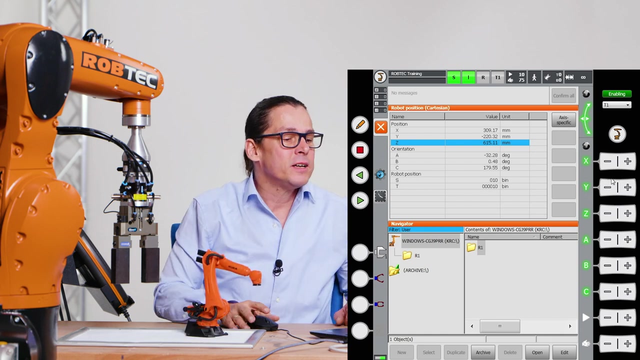 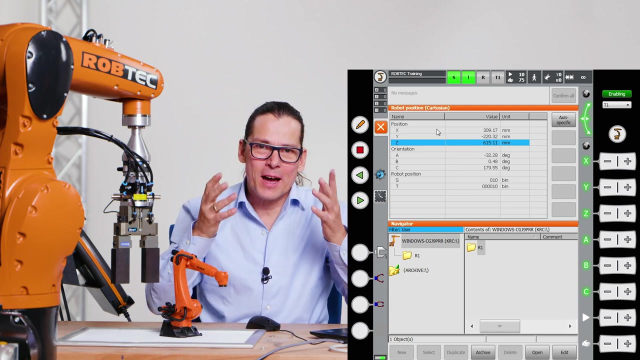 so let's give a summary. the robot has a world coordinate system. his origin is here, its origin, and the robot shows the coordinate from his actual coordinate system, which is located here, to zero, to his origin. you can see it here in the position data. so i hope you have understood.